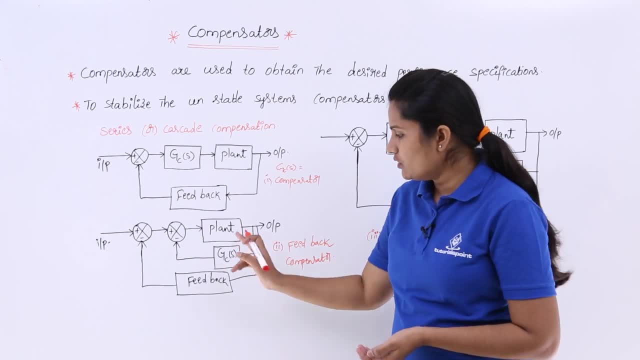 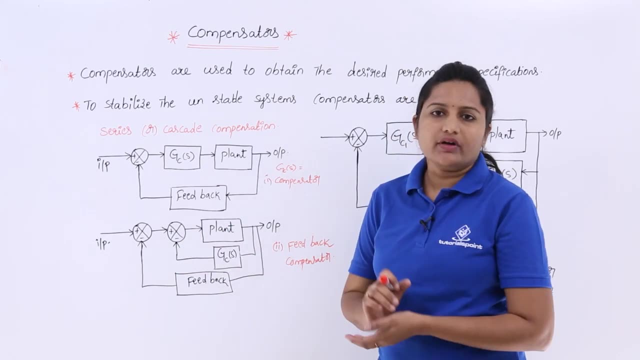 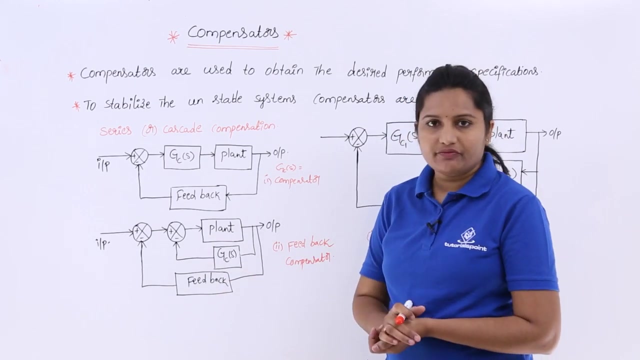 it as a feedback network. So here you can see GC of S. that means compensator is in feedback with regular gain. So this is called as feedback compensation. So this is feedback compensation network. this is cascade compensation network. So whenever your compensator is in cascade with 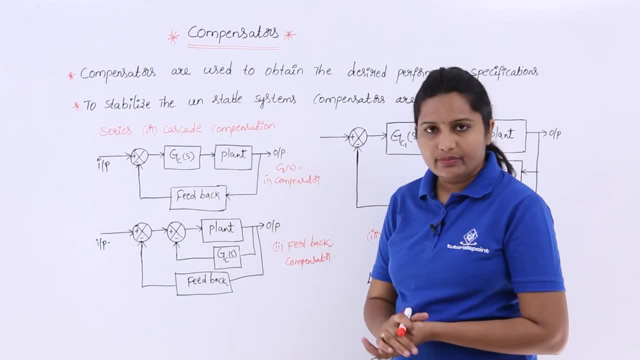 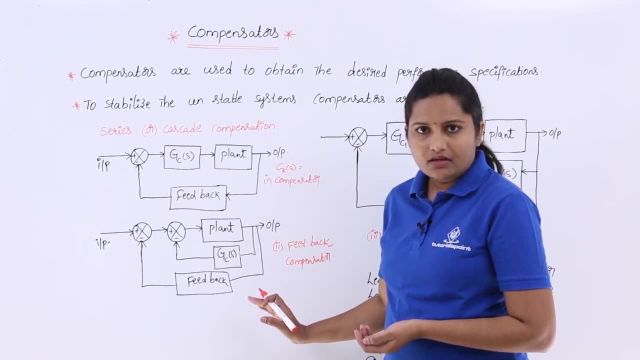 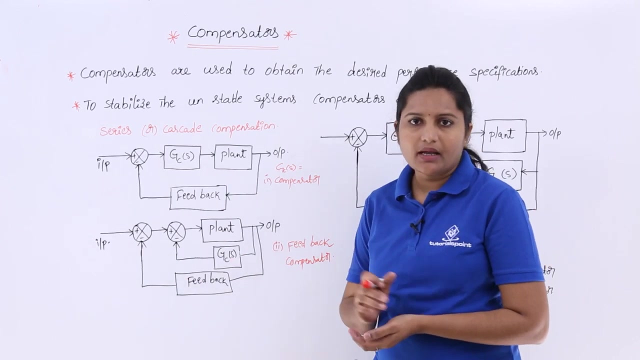 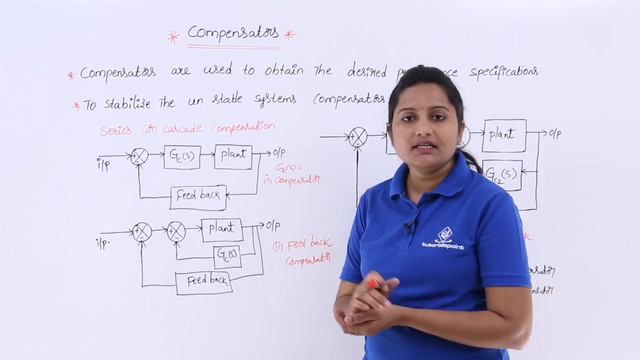 your regular gain, then that is called as cascade compensator or general compensator. Whenever you are having your regular gain with feedback, with this cascade or feedback with compensator, then we can say: this is feedback compensator. So this total network is in feedback compensation. So now coming to this diagram, 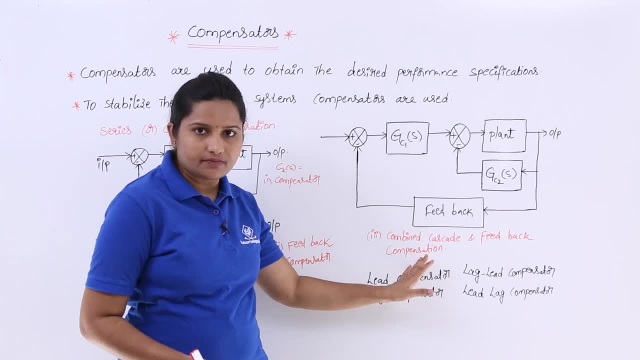 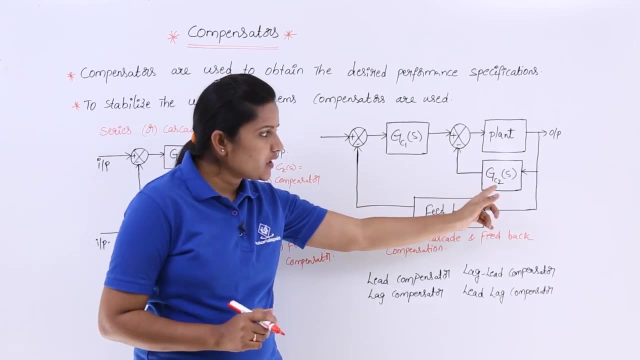 this is feedback compensation network. So now coming to this diagram, this is feedback, this combined cascade and feedback compensation. So here we are using two compensator, one in cascade network, one in feedback network. So this total control system is called as. 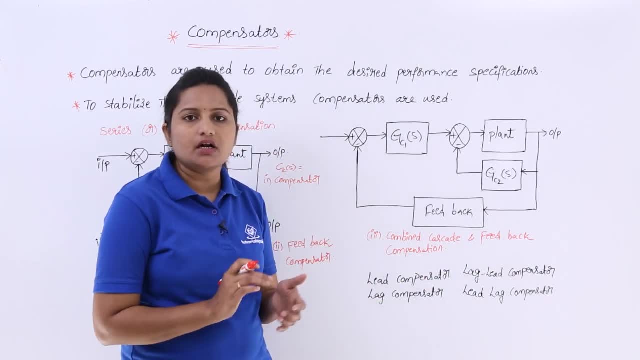 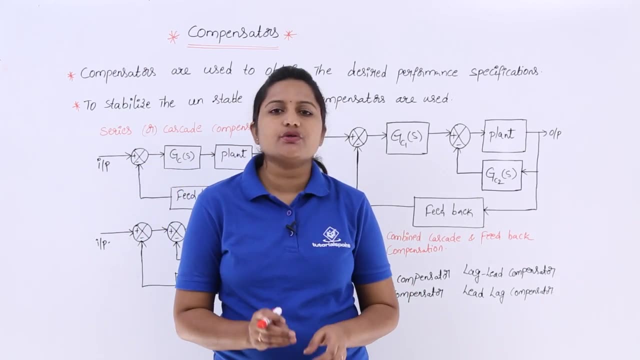 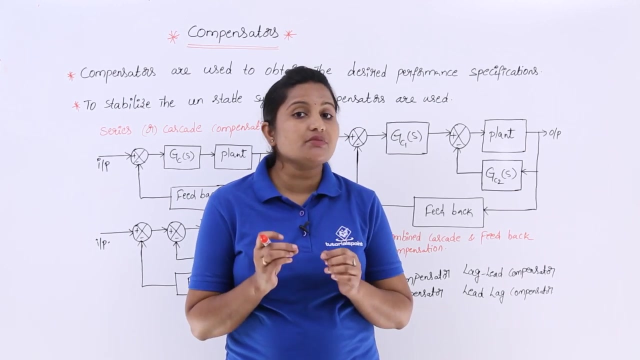 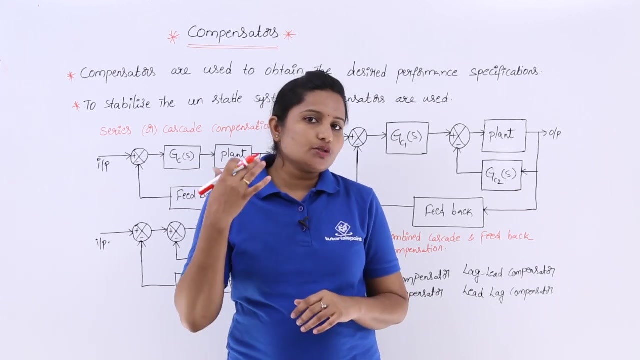 combined cascade and feedback compensation control system. So now this is about compensators generally. compensators are used to get our desired performance specifications. So in control system, especially the system, stability is our performance specification. that means required performance specification. So to stabilize the system we are going to 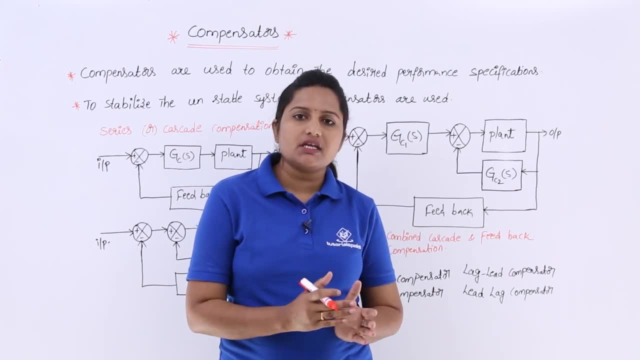 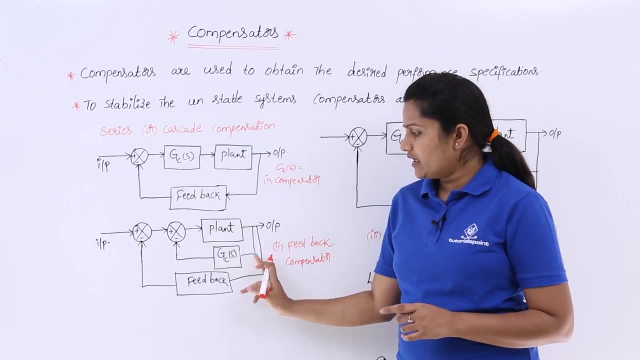